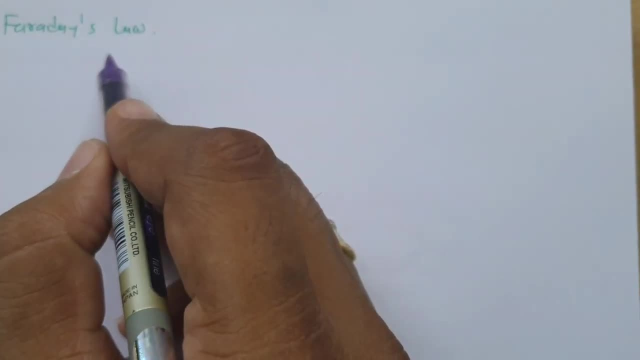 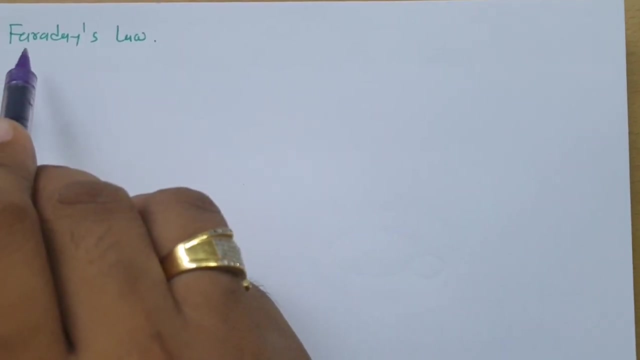 Welcome to electromagnetics playlist I. professor Hitesh Dholakia is going to explain you Faraday's law in this session. So Faraday's have done so many experiments based on time varying field and there were a few points that he has concluded. First point was see static magnetic field. 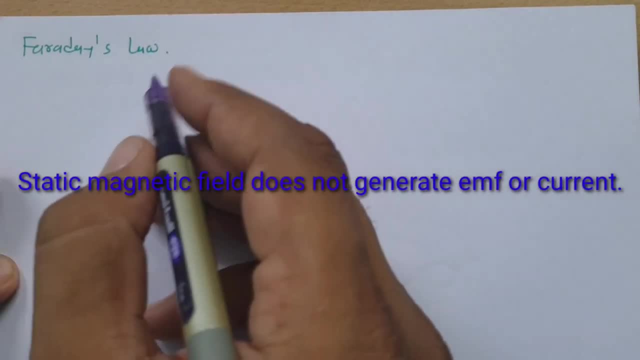 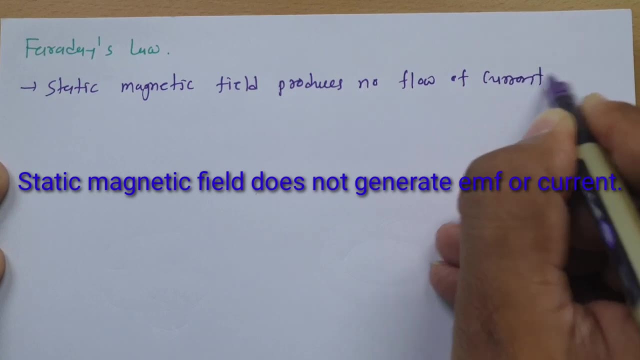 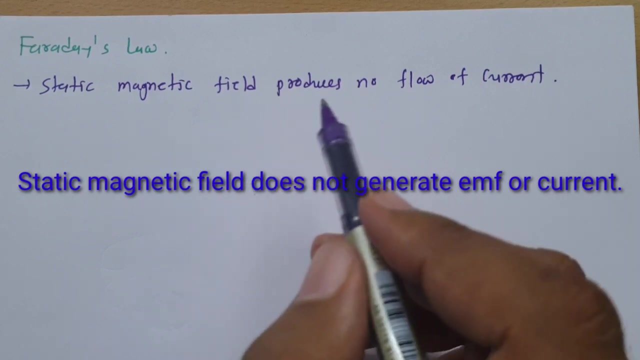 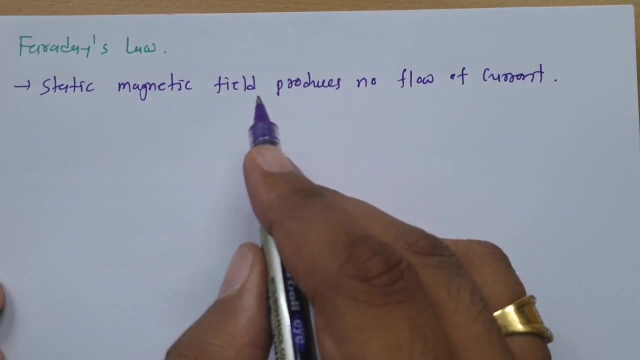 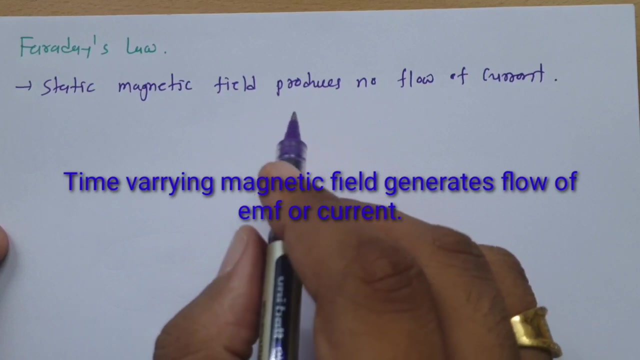 produces no current flow. So let me write all those points. So Faraday has seen, if you have static magnetic field Then that will not result any current in the circuit. but as when you change, magnetic field means time, wearing magnetic field will generate flow of current in the circuit. So we can say dynamic magnetic field or time. 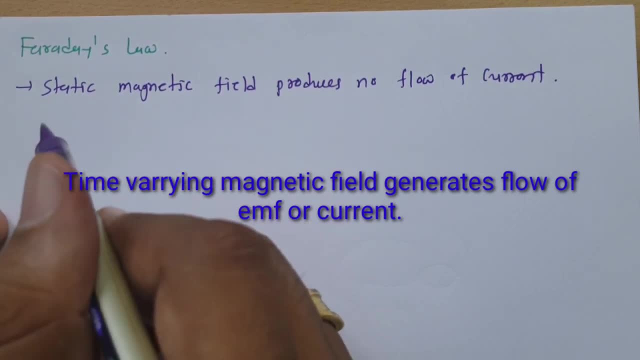 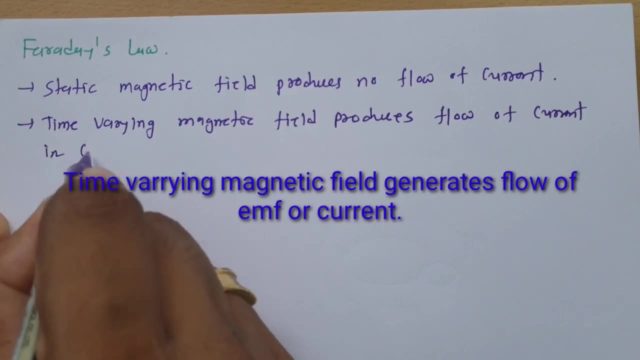 varying magnetic field field will produce flow of current in circuit. So time varying magnetic field produces flow of current in the circuit and that is happening because of induced EMF. So when you provide time varying magnetic field it will generate induced EMF. So we can say if we change flux with respect to time, then that will generate induced EMF. 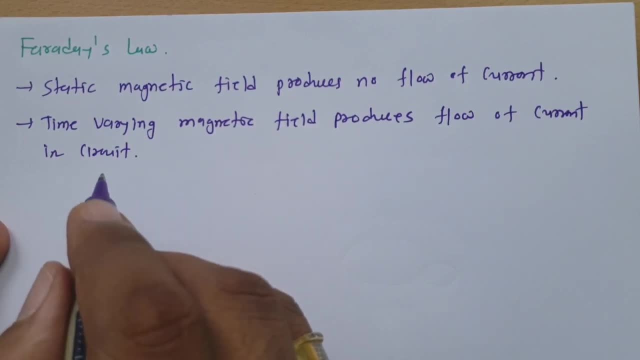 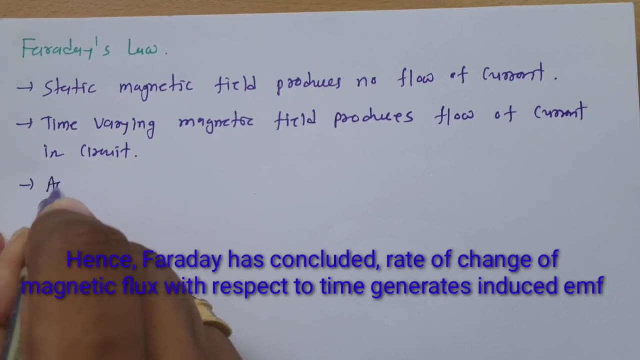 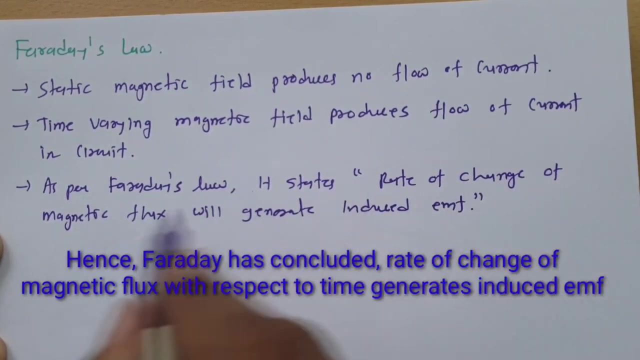 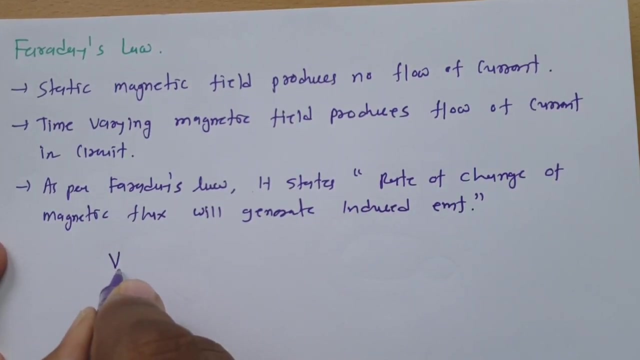 So as per Faraday's law, rate of change of flux with respect to time will generate induced EMF. So rate of change of magnetic flux will generate induced EMF. So we can say EMF means potential right. So induced EMF, that is rate of change of flux with respect to time. and here we need to place 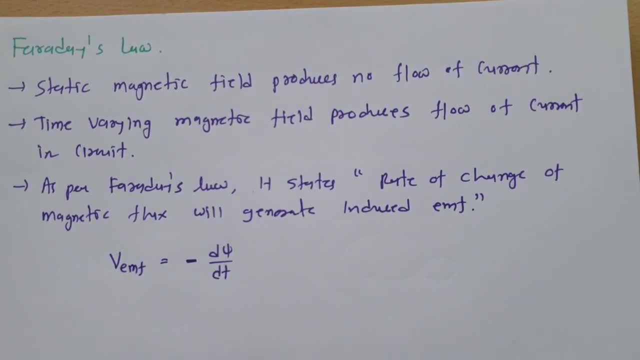 negative sign. Now see why do we place negative sign here? The reason is here: generated induced EMF current direction and direction of current generated generates magnetic field will be in opposite direction, right? So this negative sign that is due to EMF current magnitude and time varying magnitude is there. 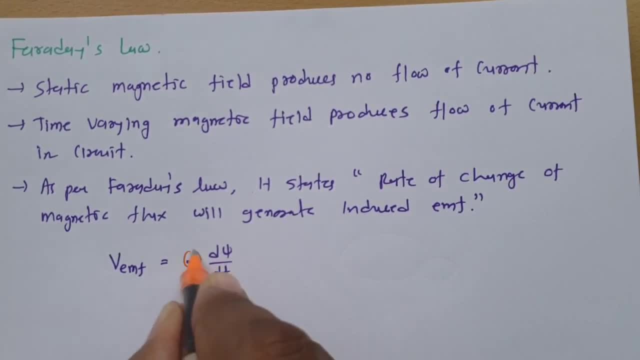 in opposite direction. So the direction of current due to EMF, see this negative sign. let me mention that this negative sign is due to EMF current Induced EMF, right induced EMF current direction and time varying direction. magnitude direction is opposite. 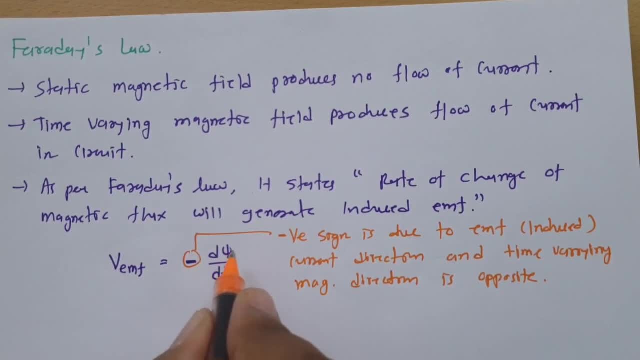 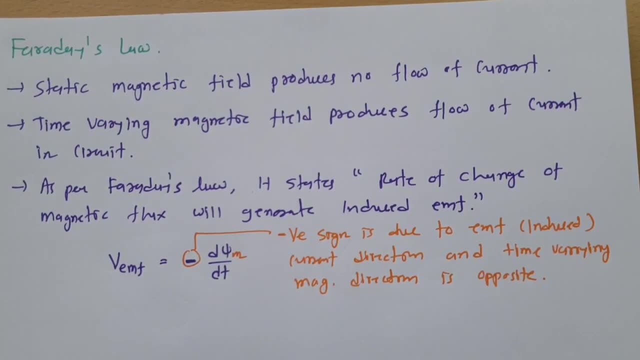 So induced EMF, that is minus of rate of change of magnetic flux with respect to time. And I have already explained what is magnetic flux. So if we place magnetic flux here, So magnetic flux is integration BDS, right, So we can say induced EMF. that is this. 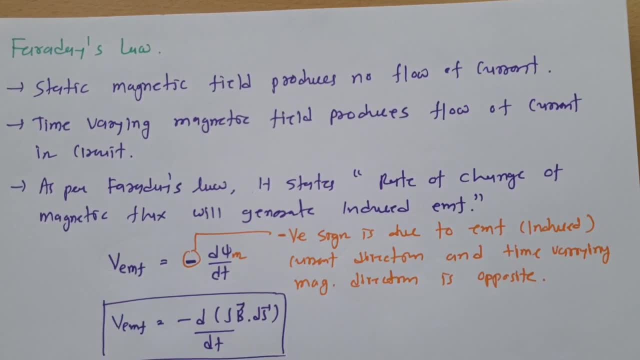 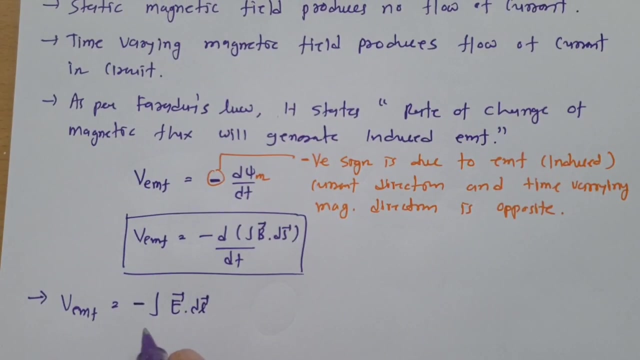 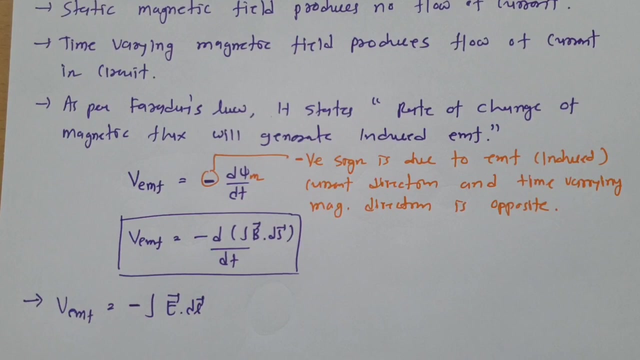 Now I have already explained you the basic definition of potential. right? So the basic definition of potential as per electric field, that is, and that is minus of integration, EDL, right So basic definition of potential, that is line integration of electric field. and here, negative sign that we used to keep. 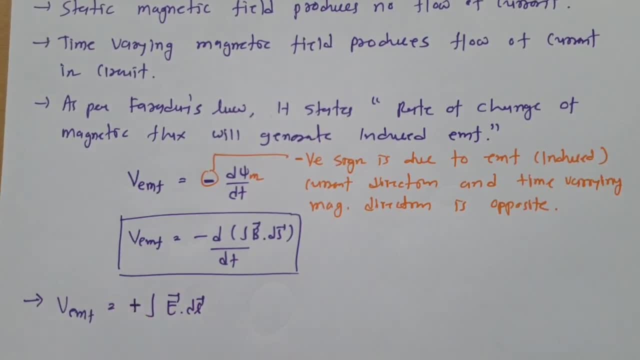 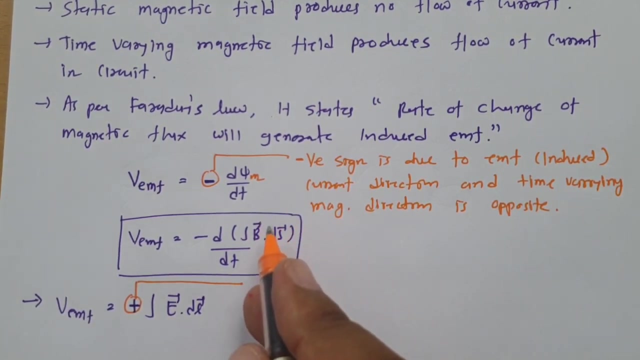 But here I need to consider this as a positive sign. Now why do I consider positive sign here? The reason is: here we consider work done on charges, So as if you calculate work done on charges, then that has to be considered positive. Why the reason is here we are doing work done on system to have change in magnetic flux. 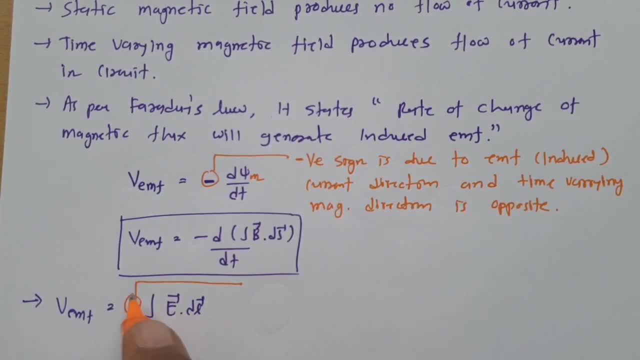 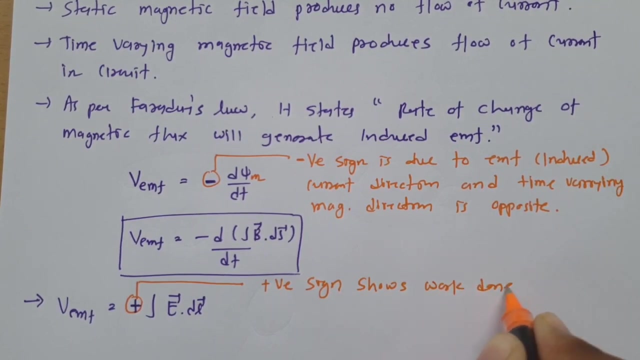 right. So here we do work done on charges. that's why we need to consider this sign as a positive. So positive sign. So here that is due to We calculate work done on charges, right. So now we have these two formula, we can compare it. 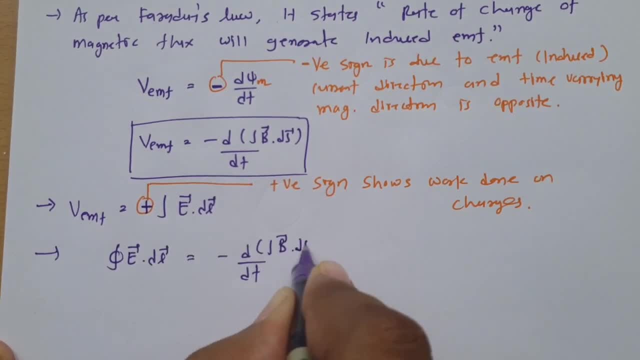 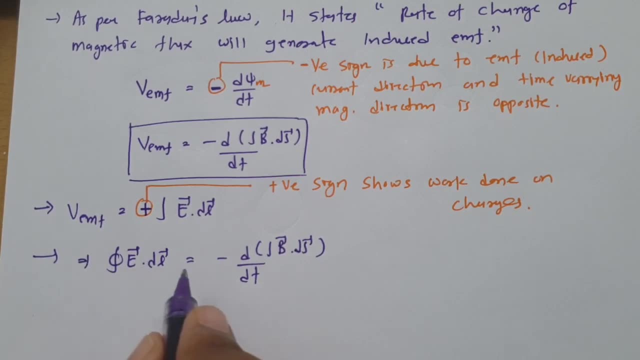 So let us compare Right Now. I have already explained you Line integration of electric field. for enclosed loop that is zero. But that is for static field right. For time varying field it will be integration. line integration of electric field that is equals to minus d by dt of surface. integration of magnetic field. 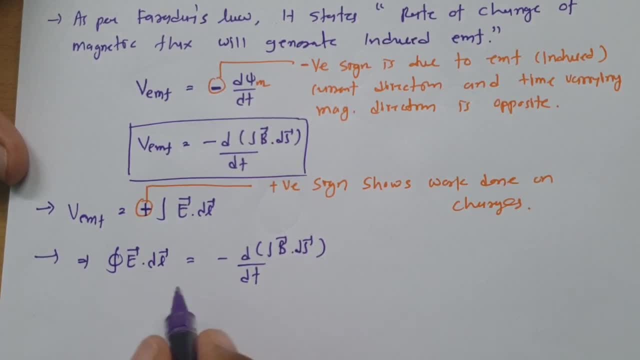 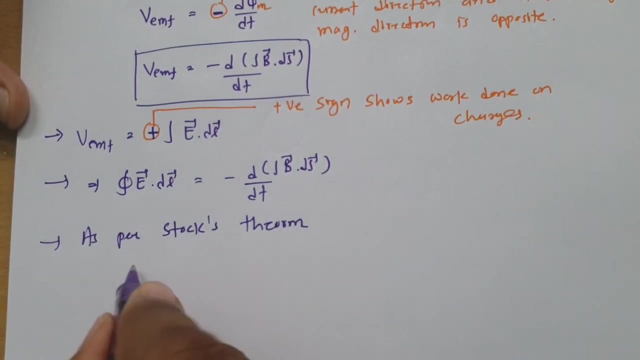 And see now, if I want to resolve this, then all I need to do is I need to apply stocks theorem. So stocks theorem, That translates Line integration into surface integration right. So as per stocks theorem, We can say line integration of electric field over closed path. 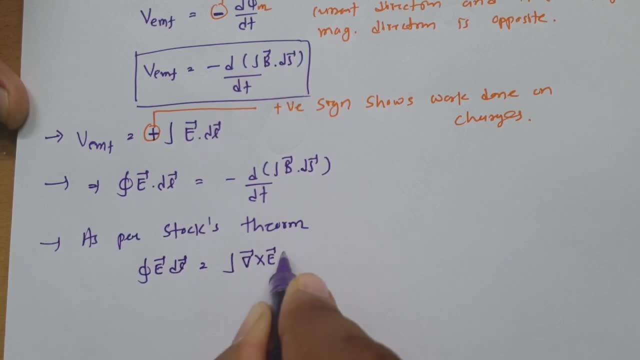 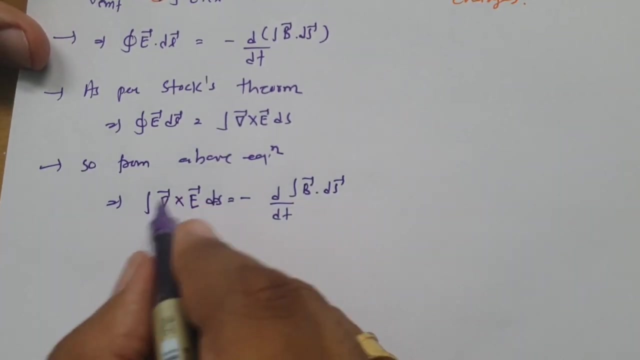 That is curl of electric field over surface integration, right. And if you Place this In this above equation, Then So now you can see this equation right and at both of the side there is surface integration, So we can cancel surface integration. 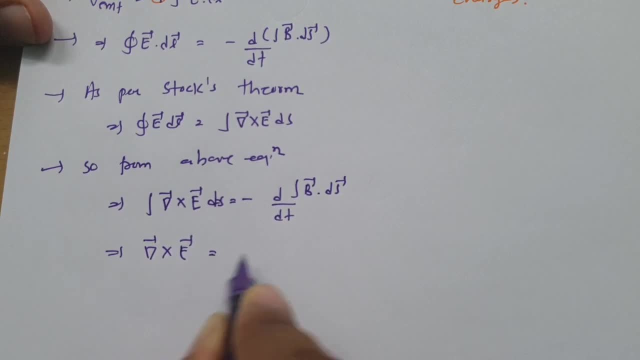 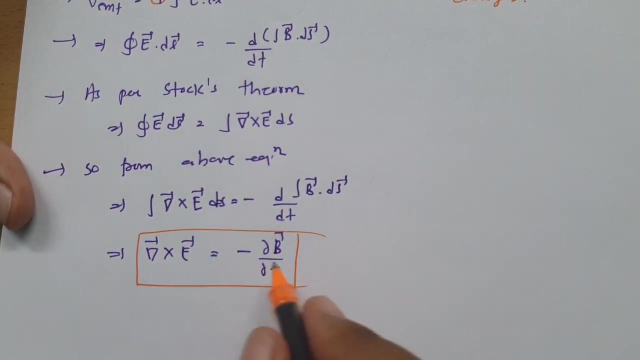 And we can say: this equation that is further simplified as del cross e is equals to minus del b by del t, Right? So this is what Maxwell's second equation for time varying field, right? So we can say: this is what Maxwell's second equation for time varying field. 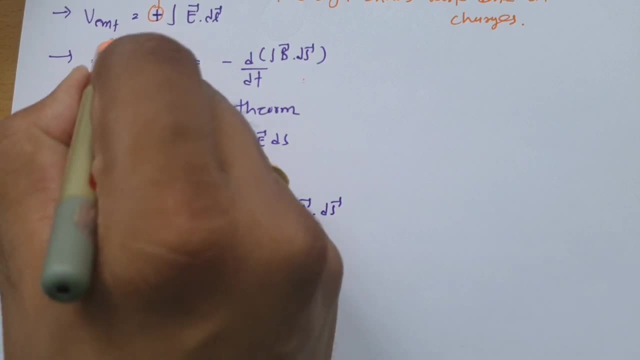 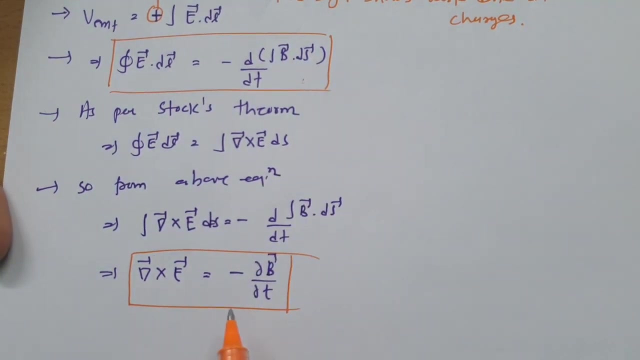 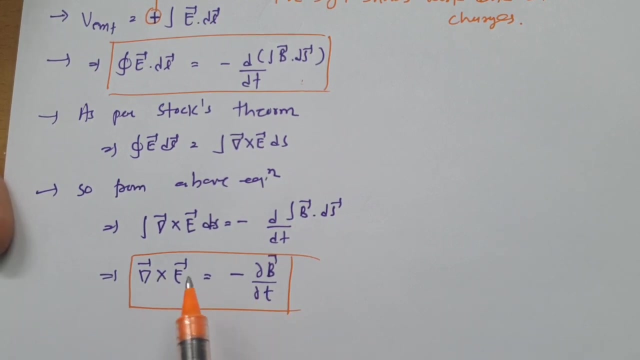 And this equation, that is Maxwell's second equation with integral form for time varying field, right. So we have seen that Maxwell's equation for A static Field, Right, But for time varying field Del cross e, that is, equals to minus del b by del t. 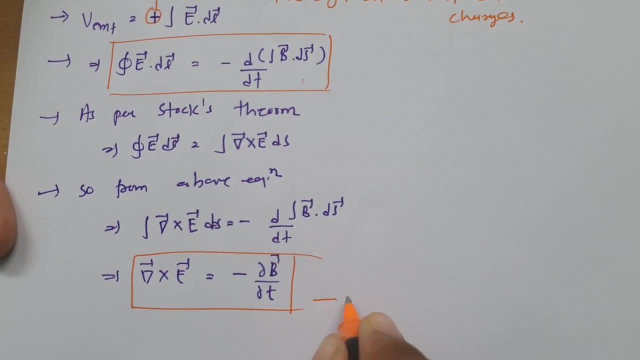 That comes from Faraday's law. So here See, if I say this is equation b, This is equation a, Then equation a And b, That is there, With Maxwell's Second Equation, Del cross e. That is there. 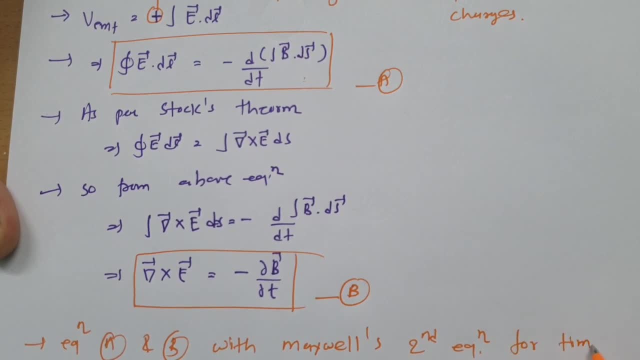 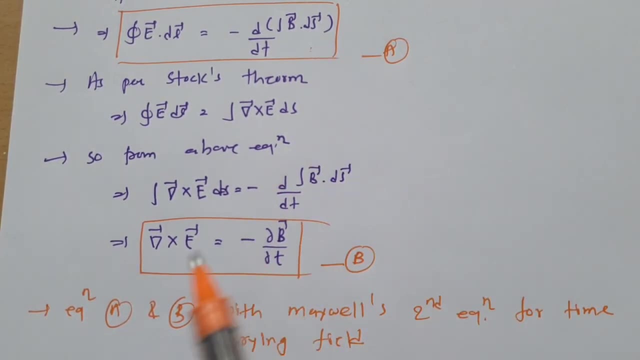 With Maxwell's Second Equation For Time varying Field. So we have already seen Maxwell's second equation, but that was for static field. now, based on Faraday's law, we can derive Maxwell's second equation for time varying field. So that is, del cross e is equals to minus del b by del t, right. 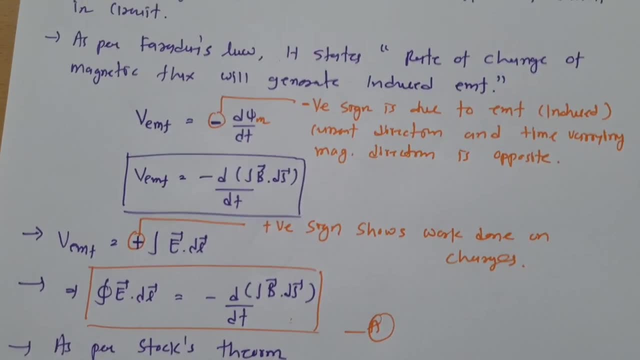 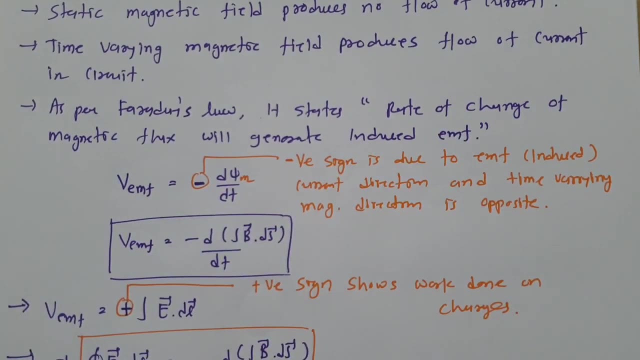 So ultimately, based on Faraday's law, we can understand so many things. See first is rate of change of magnetic flux will generate Induced EMF. So there are so many ways by which we can change magnetic flux. One is by changing position of magnet. 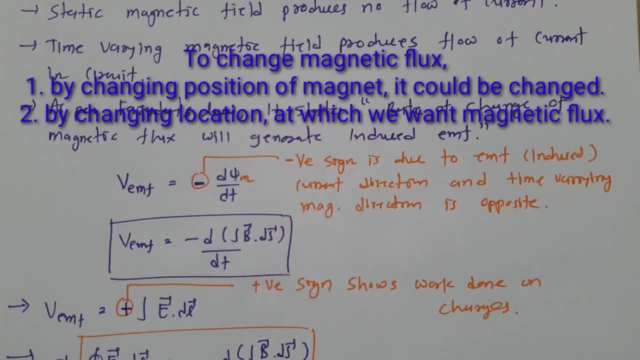 Second is by changing location at which we want to change magnetic field. Right, So there are. There is one method where, by having mechanical motion, we can provide change in magnetic flux. Now see second way. that is what we can generate, it by having. 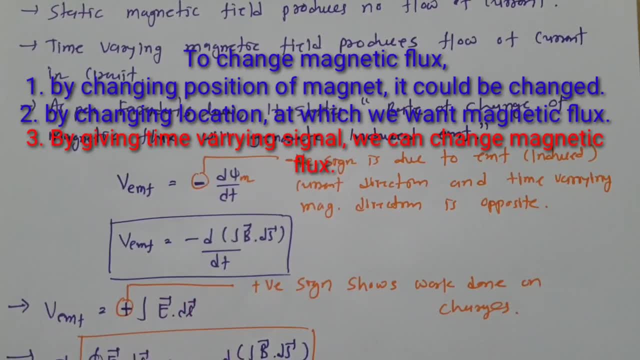 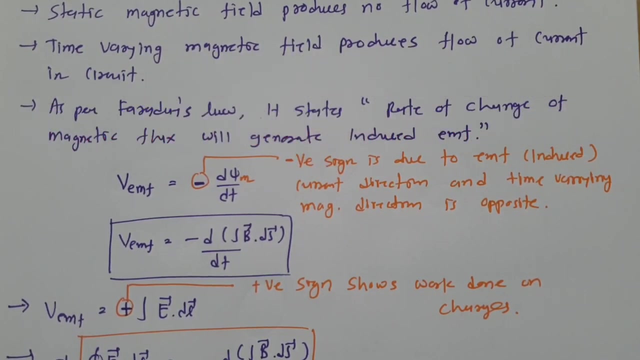 Signal. So So if you give signal which is changing with respect to time, So for high frequency signal, magnetic field will change with respect to time And that change in magnetic field will generate induced EMF. So there are so many applications which is there with Faraday's law. 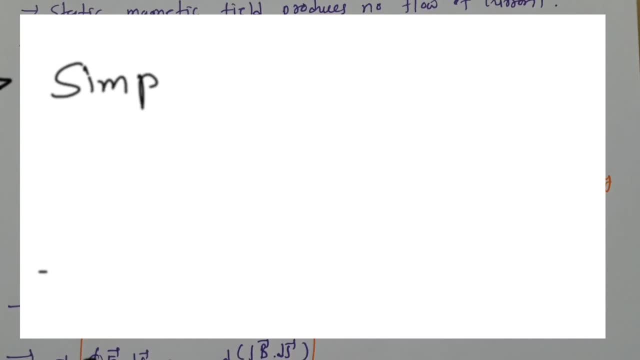 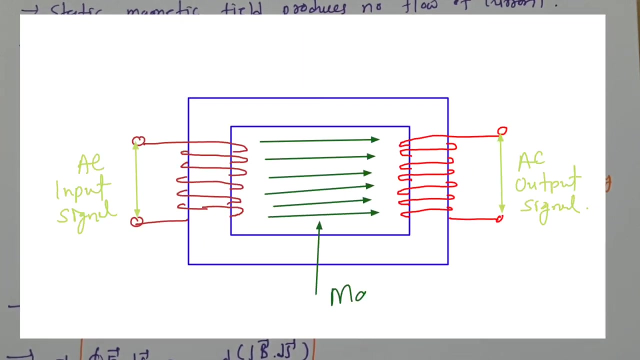 You might have seen one basic application that is transformer. So in transformer all we do is we provide AC signal to Primary winding and because of signal is AC signal flux will get leakage to secondary and that flux will change with respect to time and that will generate induced EMF in. 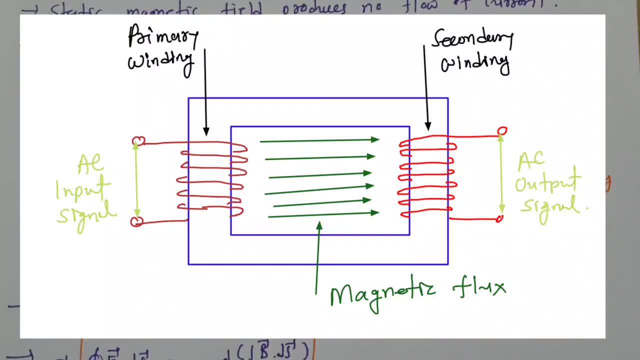 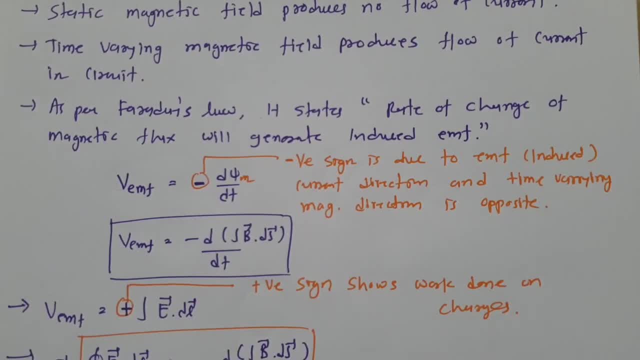 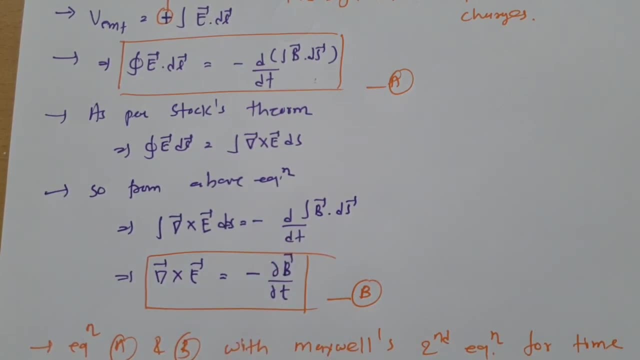 secondary winding. So this is one basic application of Faraday's law In electromagnetics. there are so many applications. like by using Faraday's law we can understand there is a relation in between electric field and magnetic field for time varying field. So 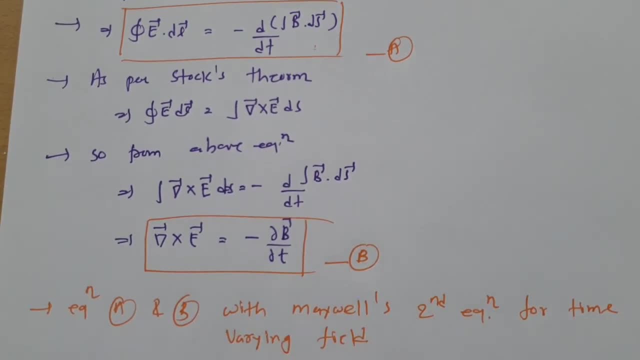 Faraday's law states second equation of Maxwell for time varying field and it gives you relation in between electric field and magnetic field. You see, this Curl of electric field is equals to minus of rate of change of magnetic field. So as if you change magnetic field there is electric field and as if you change electric